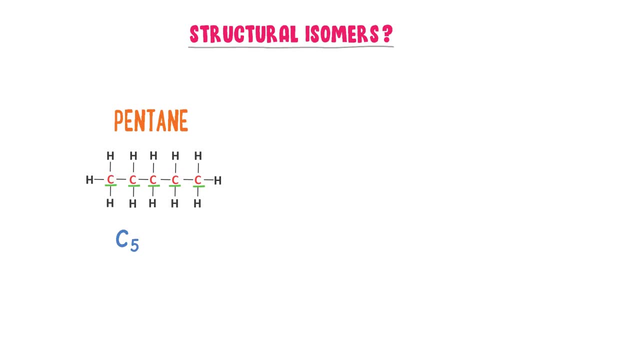 atoms. Now let me count the hydrogen atoms: 1,, 2,, 3,, 4,, 5,, 6,, 7,, 8,, 9,, 10,, 11,, 12.. So there are 12 hydrogen atoms. Hence the molecular formula of a pentane is C5H12.. Now again, 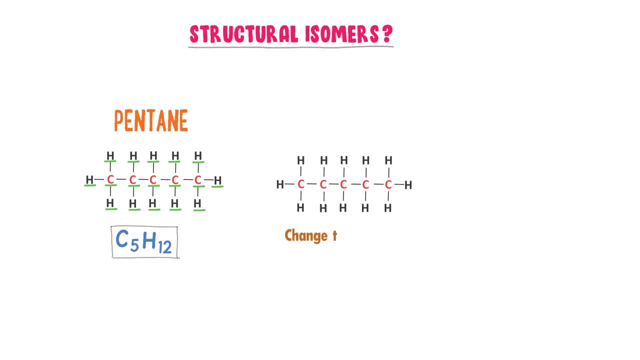 consider this pentane. I am interested to change the structure of this pentane. Can you guess that? How can I change it? Well, there is one way: I should cut the long chain of carbon atoms. I mean changing the arrangement of carbon atoms. So I cut this fifth carbon. 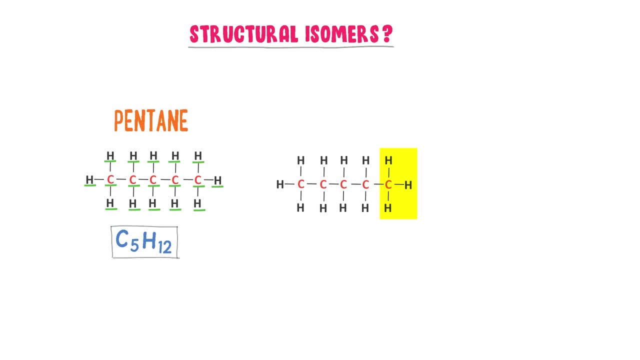 along with its three hydrogen atoms. Secondly, I cut this hydrogen of second carbon. I will shift their positions. I place this carbon, along with its three hydrogens, on this second carbon and I place this hydrogen instead of this carbon. After changing their respective positions, I get this type of structure. 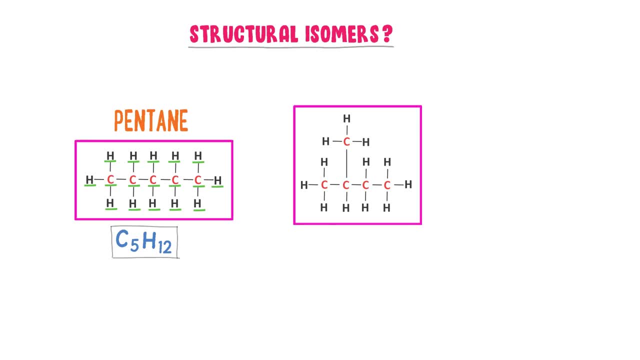 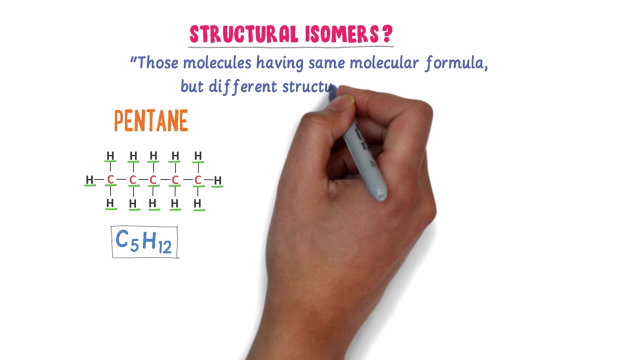 of pentane, Although these both structures are different, but they have the same molecular formula, C5H12.. Therefore we define structural isomers as those molecules having the same molecular formula but different structural formula are called isomers. Let me repeat it. 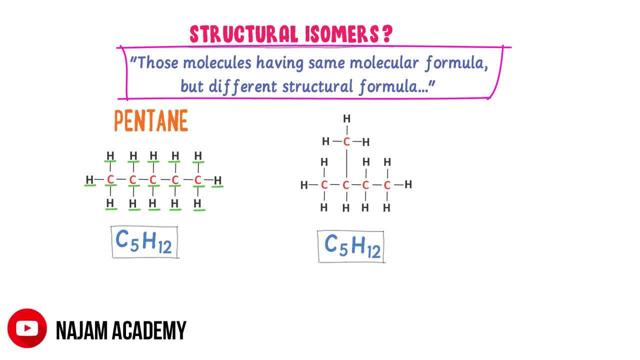 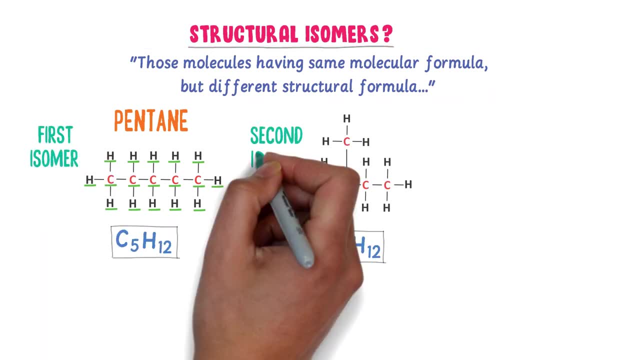 Those molecules having same molecular formula but different structural formula are called isomers. So this is first isomer of pentane and this is second isomer of pentane, But they have same molecular formula, C5H12.. Secondly, we therefore call them structural isomers. 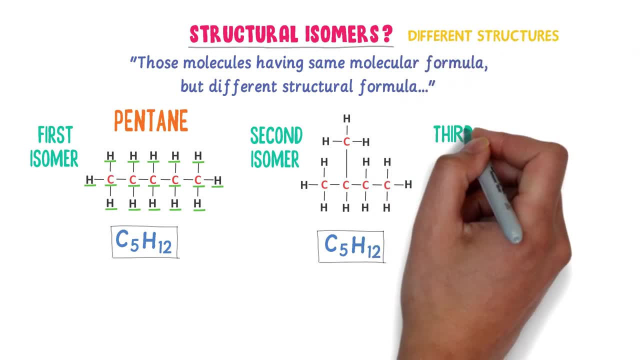 because they have different structures. Also, we can draw third isomer of pentane by changing the arrangement of carbon atoms like this. Still we can see that there are five carbon and twelve hydrogen atoms present in it. So again, its molecular formula is C5H12, but its structure is totally different. 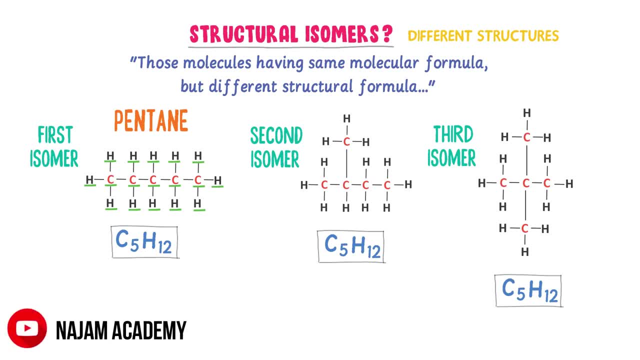 from these two isomers. So this is the third isomer of pentane. Therefore, note it down that the isomers are those molecules which have same molecular formula but different structural formula. I hope that you have learnt all about the structural isomers.